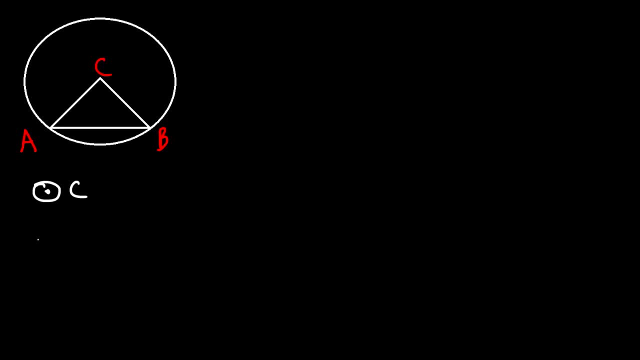 So our goal is to prove that triangle A, C, B is isosceles. So how can we do this? Well, let's start with a two column proof. On the left side we're going to put statements and on the right side, reasons. 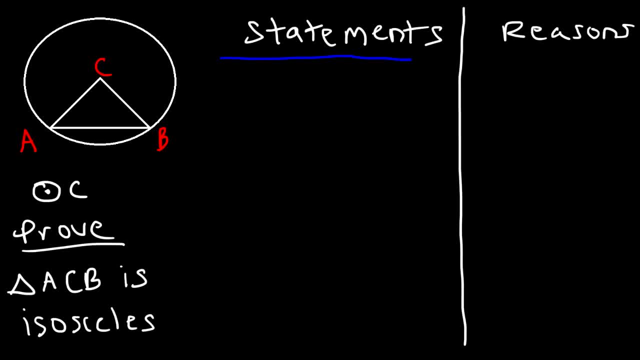 So let's start with the first statement, That point C is the center of the circle, And that's given. Now number two: what else can we see If we know C is the center? what else do we know? What do we know about segments A, C and B? C, A, B is a chord. 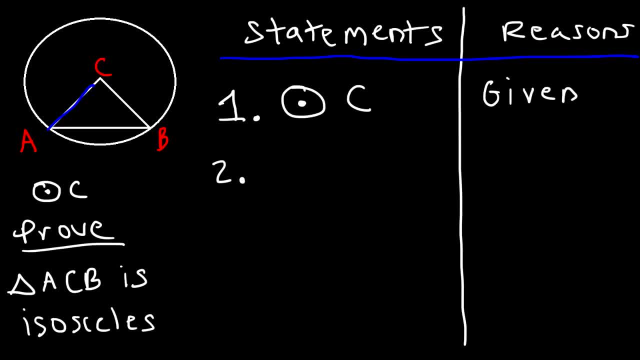 But A, C and C- B. that represents the radius of the circle. The radius is the distance between the center of the circle and any point on the circle. Points A and B are on the circle, So therefore we could say that segment A- C is congruent. 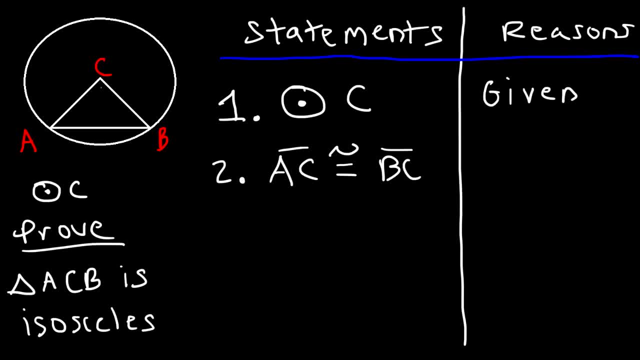 To segment B, C, And the reason for that? they both represent the radius of the circle. So what can we put in the second column? What's the reason for this? All radii of a circle are congruent. That's the reason. 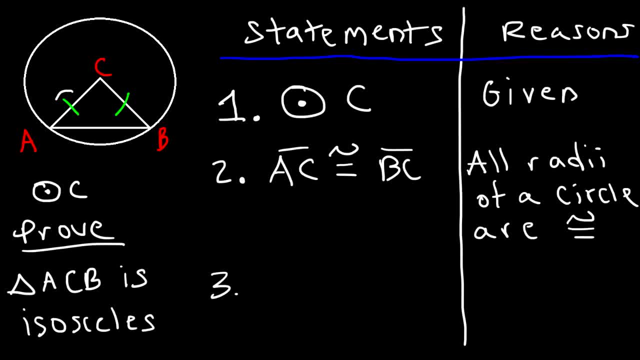 So now, because we have a triangle where two sides are the same, we can now say that this is an isosceles triangle. So triangle A, C, B is isosceles. Now what should we write in the second column? 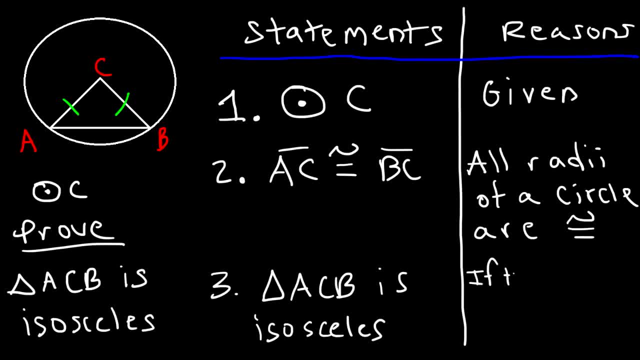 We could say that if two sides, if two sides of a triangle are congruent, then the triangle is isosceles, And so that's it. That's how you can prove that this particular triangle is an isosceles triangle. 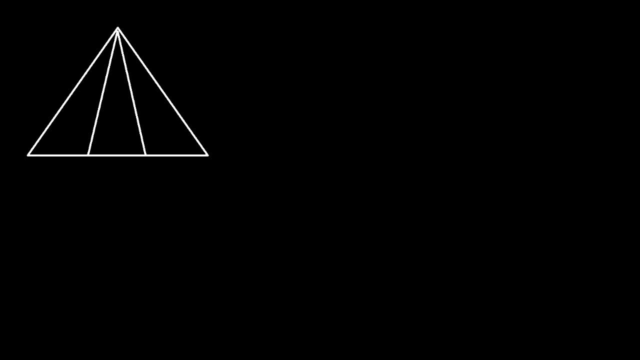 Now let's try another example. So this one is going to involve a lot more steps. So let's call this A, B, C, D and this is going to be point E. Now in this problem, we're given that segment EB is congruent to segment EC. 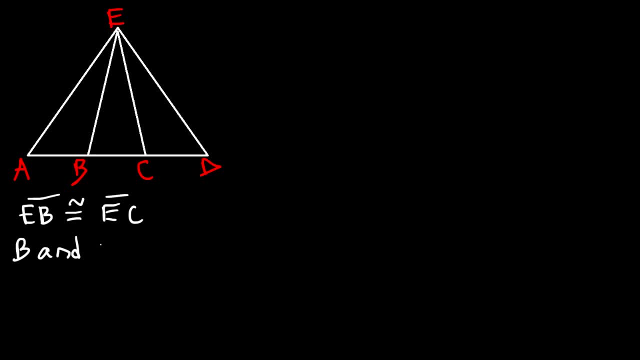 Now we're also given that B and C- that's points B and C- they trisect segment AD. And finally, angle ABE is congruent to angle DCE. So our task is to prove that triangle AED is an isosceles triangle. 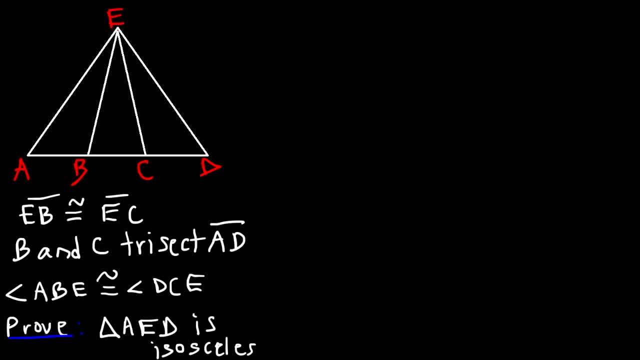 So feel free to work on this problem. if you want, Pause the video and then write out the two-column proof And then, when you're finished, just unpause it to see if you have the right answer. Now, before we begin, let's see if we could plan out some steps. 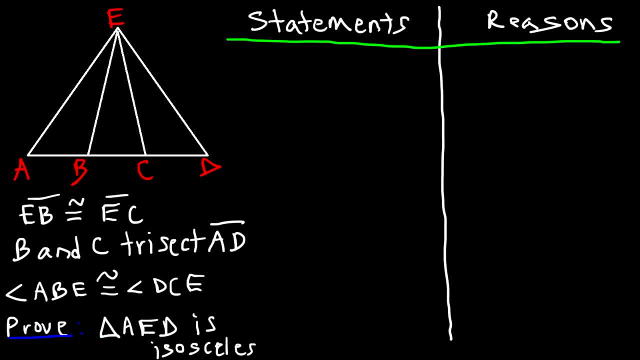 So our goal is to prove that triangle AED is isosceles. So this is triangle AED. In order to prove that that particular triangle is isosceles, we need to show that two sides are congruent: Either AE equals ED or AE equals AD something. 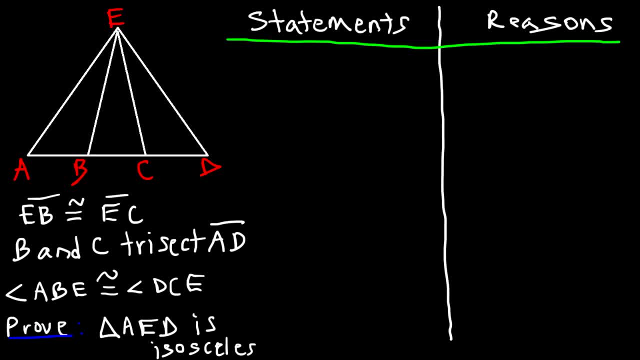 So we've got to prove that two sides are congruent. In order to prove that those two sides are congruent, What we could do is prove that triangle AEB is congruent to triangle DEC. If we could prove that those two triangles are congruent, then any part of those two. 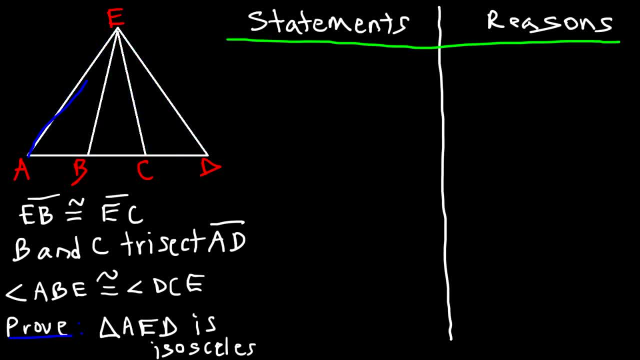 triangles are congruent, including their sides, So let's try to do that. So let's start with what we're given: EB is equal to EC, so let's write that in the first column. So segment EB is congruent to segment EC. 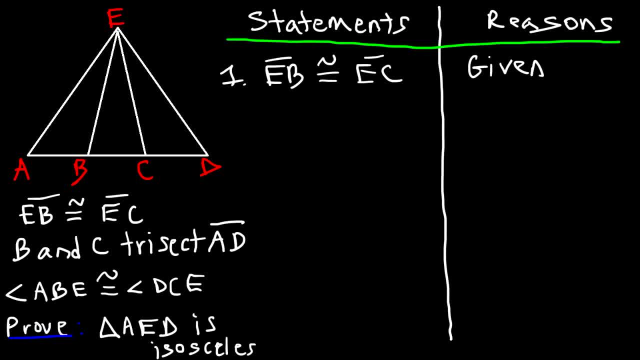 And that's just that's given to us, And let's mark it on the diagram. So this is EB and this is EC. So that's a step in the right direction. Now let's move on to our second given statement, And that is point E. 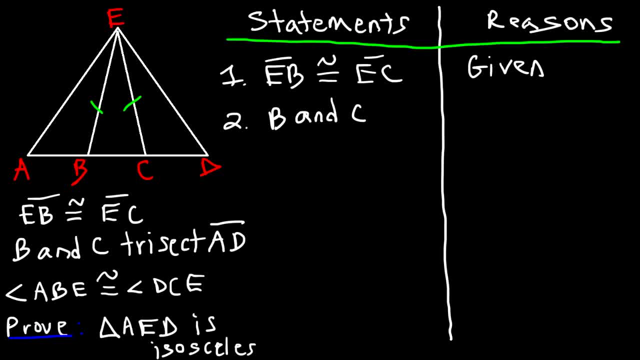 Points B and C trisect segment AD, And that's given to us as well. Now, if points B and C, if they trisect this segment, what does that mean? Well, a segment bisector is basically a point that splits the segment. 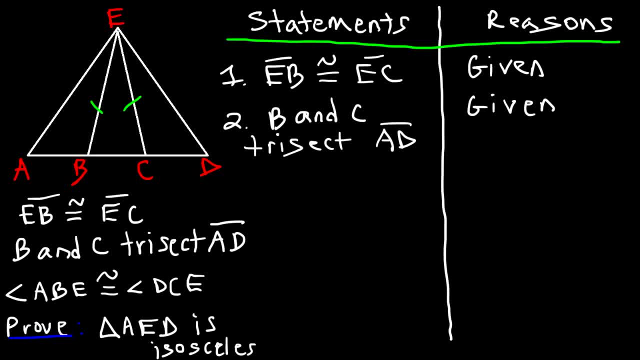 A segment into two congruent parts. So if two points trisect a segment, that means that they split the segment into three congruent parts. So that tells us that AB is congruent to BC and BC is congruent to CD. So all three of those sides. 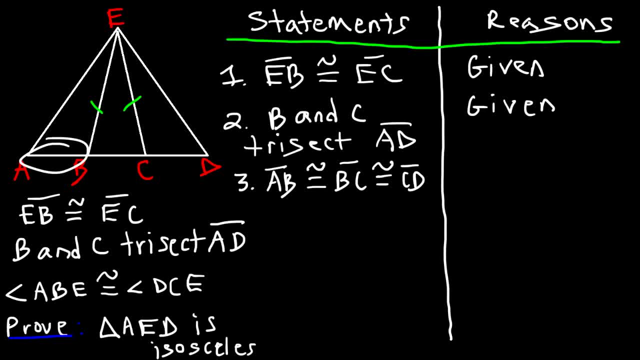 So AB, BC and CD, they are congruent to each other. So what can we write for the reason for step three? Well, we could say it's based on the definition of a segment trisector as opposed to a segment bisector. 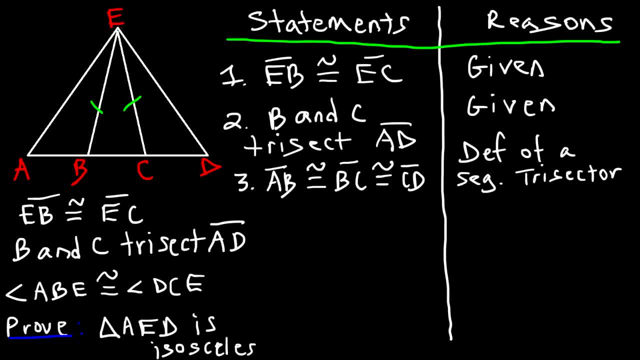 Now I'm going to need to make some more space, So what I need to do is just get rid of this stuff, because I already have it in the statements column, So let's delete that. And now let's move on to step four. 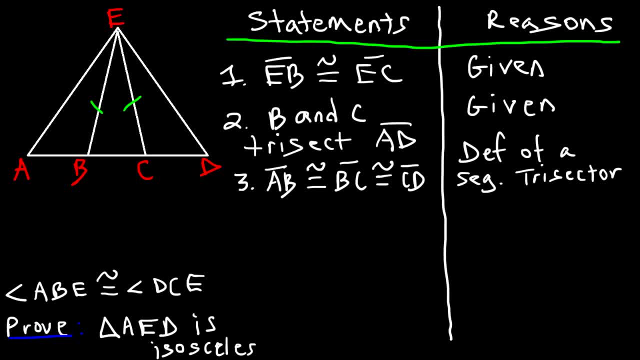 But before we do that, let's mark a few details on the diagram. So what we really need is AB and CD. That's what we got to show, because our goal, remember, is to prove that these two triangles are congruent And BC is outside of those two triangles. 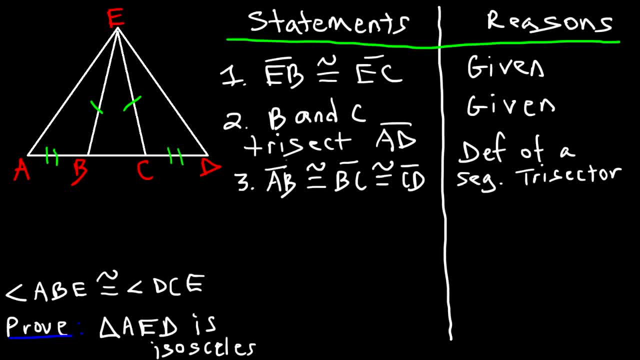 So I'm going to mark that AB is congruent to CD, which we do have here Now. I only need to prove one more feature of these two triangles. If I can prove that something else is congruent, then I could state that those two triangles 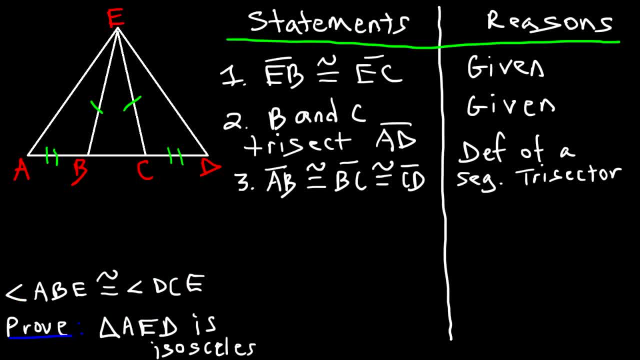 are congruent, And we're given this. So in statement four we could say that triangle, or rather angle, angle ABE is congruent to angle DCE, And so that's given to us, And now let's mark it in the graph. 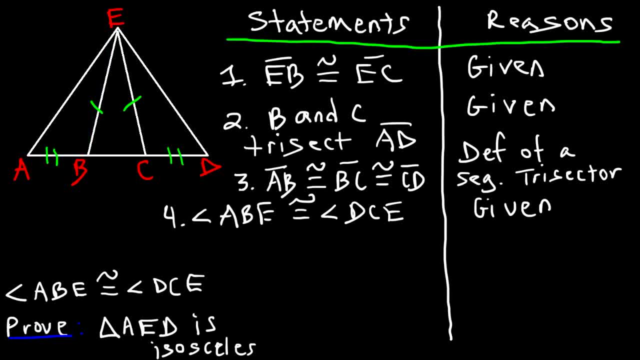 So this is ABE And here is angle DCE. So ABE is congruent to DCE. 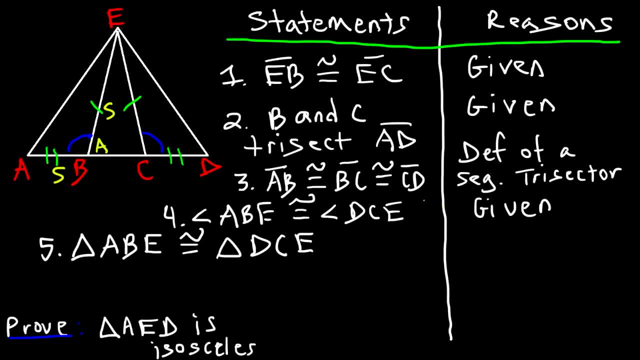 SAS postulate the two triangles are congruent, and so for the first side, if we go in order, it was based on statement 1- EB is congruent to EC. now the angle was based on statement 4, and then we prove that these two sides are congruent and that was based on statement 3. 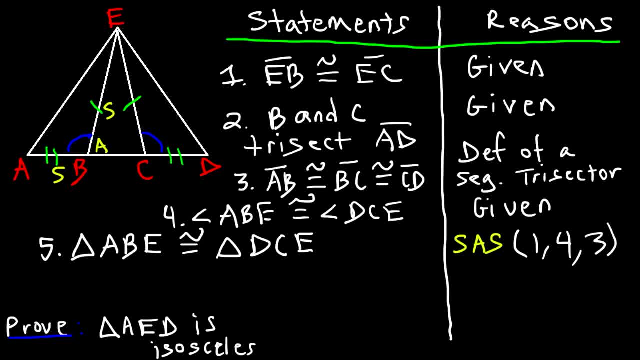 so the reason is SAS statements 1, 4, 3 in that order, in the order of SAS, not necessarily in a numerical order. so now, what else can we say, now that we've proven that the two triangles, a, B, E and DCE, are congruent? so what statement can we make at this point? 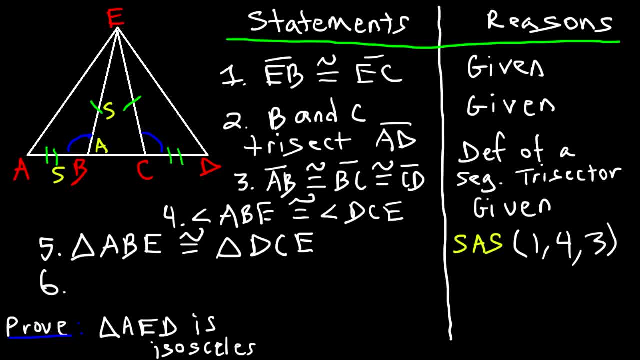 if two triangles are congruent, then all of their corresponding parts are congruent. so we can now say that segment AE is congruent to segment ED. so AE is congruent to D and a reason: CP, CTC, corresponding parts of congruent triangles are congruent. 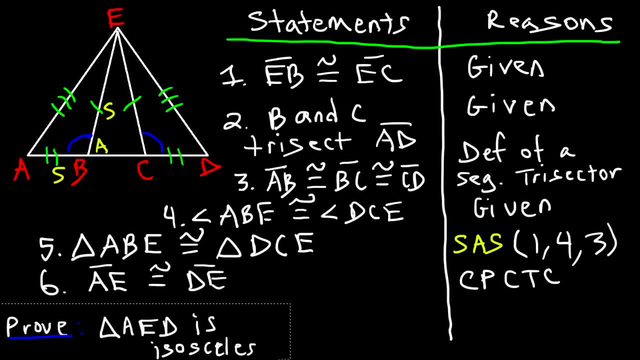 so now that we've proven that those two sides are congruent, we can go one step beyond CP, CTC, and so we could prove that triangle a ED is an isosceles triangle, and the reason for that is the same as the last example. let's see if I could fit in here. 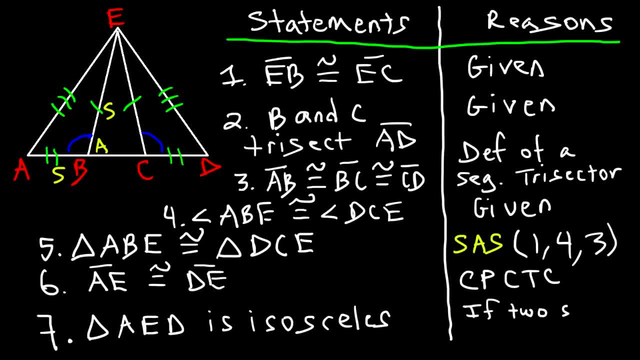 so if two sides of a triangle are congruent, then the triangle is an isosceles triangle and that's it. so now you have two examples on how to prove that a triangle is a softly. the basic idea is: your goal is to prove that two sides are congruent. 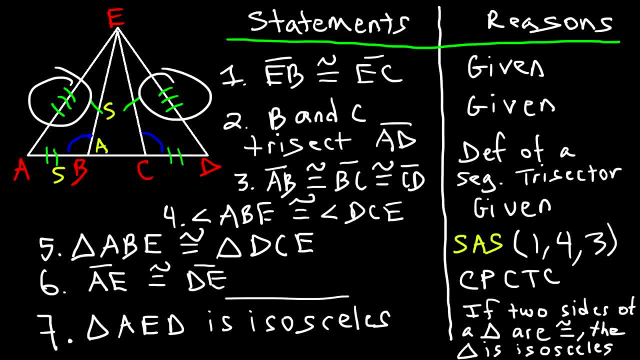 once you have that, then you can make the final statement that that triangle is isosceles, and you can use the same reason if you want to. so now you know how to prove if a triangle is isosceles. now let's look at one more example. so 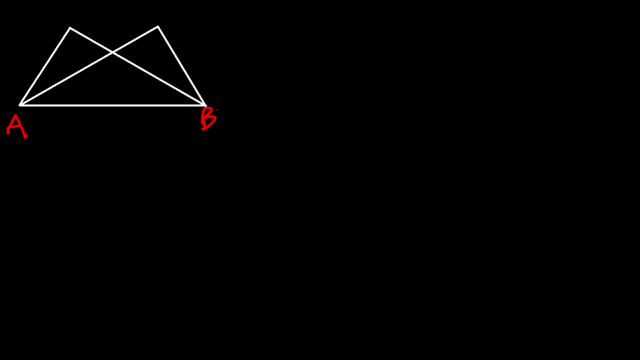 let's say that this is point a, B, C, D, and here we have E. now Now in this problem, let's mention one more thing. let's say: this is angle 1 and angle 2.. So we're given that angle 1 is congruent to angle 2.. 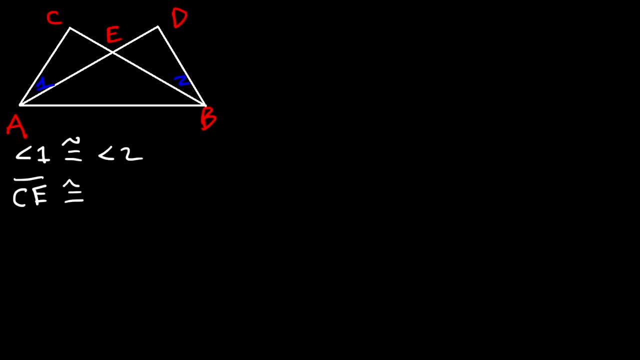 In addition, CE is congruent to DE, Prove that triangle AEB is isosceles. So let's do a two column proof, Statements and reasons, If you want to, based on the last two examples, go ahead and tackle this problem. 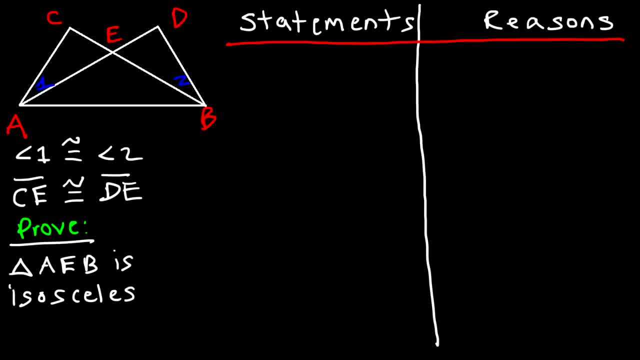 Now, before we begin, let's create a mental outline of what we need to do in order to prove that. Let's say that triangle AEB is isosceles. So what do we need to know in order to prove that that triangle is isosceles? 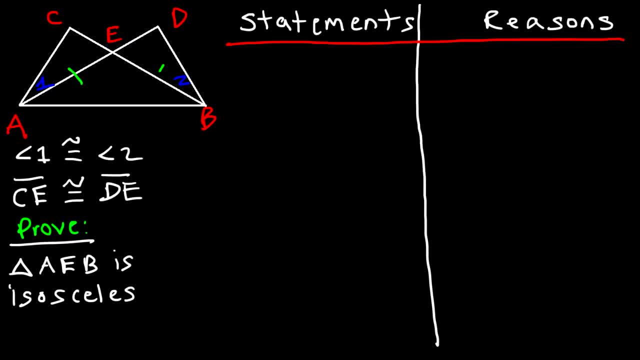 We need to show that AE is congruent to EB And in order to show that those two segments are congruent to each other, we need to show that triangle ACE is congruent to BDE. So how do we prove that those two triangles are congruent? 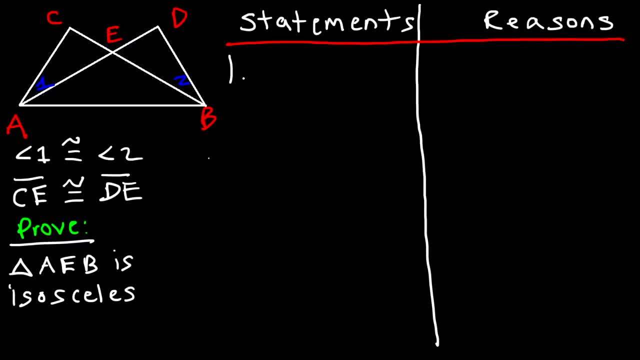 Well, let's start with statement 1.. Let me write smaller. I might need some more space. I went too far. So we can say that angle 1 is congruent to angle 2. And that's given to us And we can mark it on the graph. 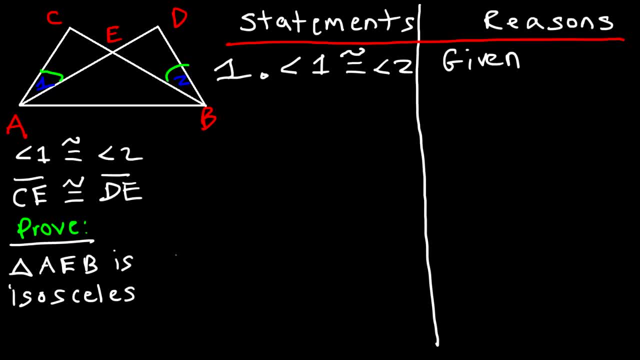 So here it is. This angle is congruent to that angle. Now let's say that angle 1 is congruent to angle 2. And that's given to us And we can mark it on the graph. Now let's go in order. 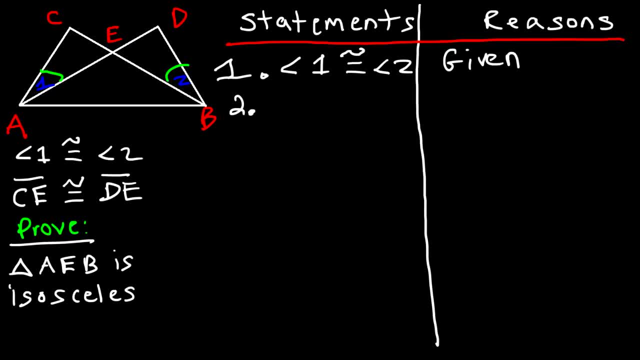 So number 2, we could also say that this angle is congruent to this angle. Why can we say that Whenever two lines intersect each other, they will produce something known as vertical angles. Vertical angles are congruent to each other. So for statement 2, we could say that: 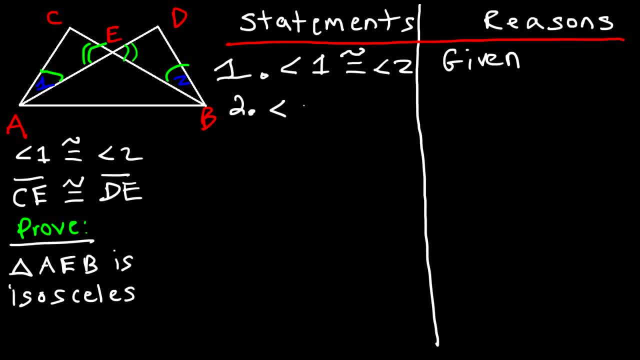 Let's see if I can fit it in here. Angle AEC is congruent to angle BED, And the reason: Vertical angles are congruent. So that's what we can say for the reason. Now let's move on to the next part. 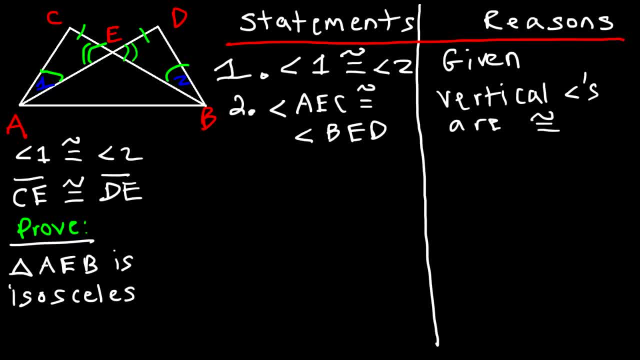 So we know that CE is congruent to ED And that simply is a statement that was given to us. So let's write given. Now we have enough information to prove that these two triangles are congruent, So let's make the statement that triangle AEC. 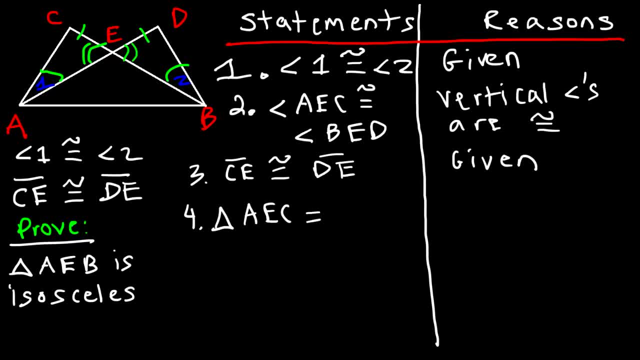 So that's this triangle. That is this triangle That is congruent to triangle BED. So this is BED. Now, what's the reason? Why can we say that those two triangles are congruent? So we have an angle, an angle and a side. 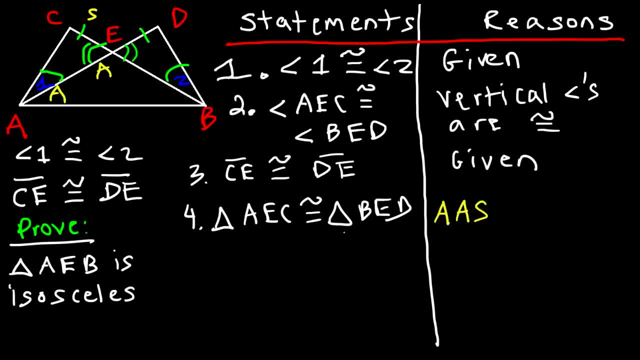 So it's based on the AAS postulate. So, starting with this angle, it came from statement 1.. And then the second angle, vertical angles, came from statement 2.. And then the third part, the side, came from statement 3.. 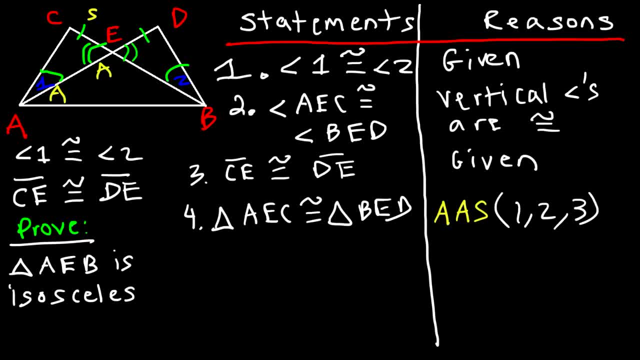 So it's based on statements 1,, 2, and 3.. Now that the two triangles are congruent, we can make a statement that their corresponding parts are congruent. So we can now say that AE is congruent to BE. 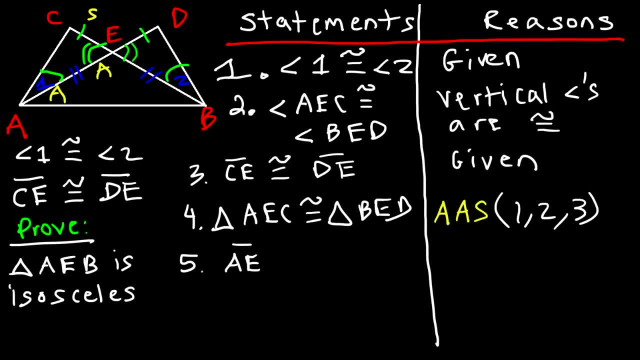 So that's going to be statement 5.. AE is congruent to BE And the reason for that is, as we know, CPCTC- Corresponding parts of congruent triangles are congruent. So now we can make the final statement.